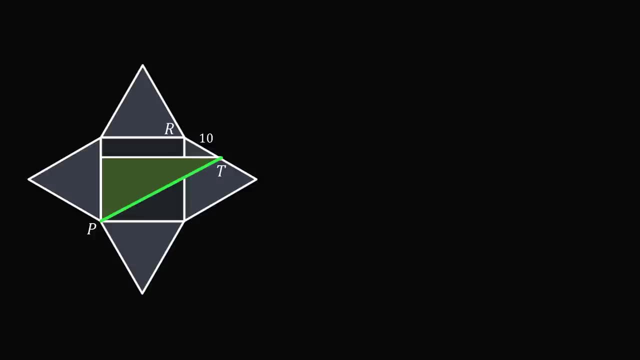 Next, each triangular face is an equilateral triangle because all three sides have the same length, So each of these angles is equal to 60 degrees. We thus have a 30-60-90 right triangle with the hypotenuse R T equal to 10.. So the shorter leg will be equal to 5, and the longer 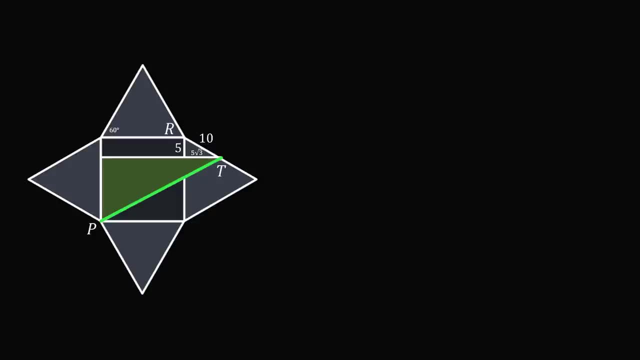 leg will be equal to 5 times the square root of 3.. To calculate the remaining distance along this side triangle, notice its length is exactly equal to the side length of the square, so it's equal to 20.. To calculate the remaining distance, we take 20 minus 5, which is equal to 15.. 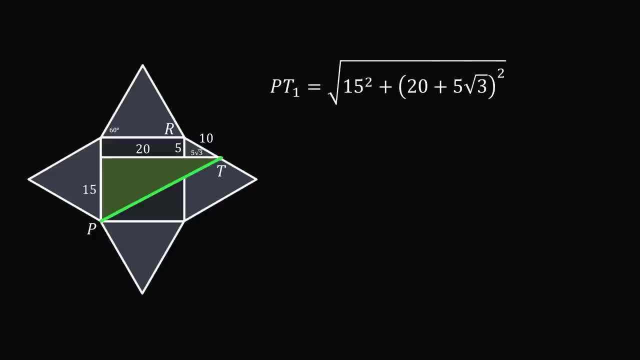 We can thus calculate that P T is equal to the square root of the sum of the squares of 15 and the quantity 20 plus 5 times the square root of 3.. So in this case, P T has a length equal to the square root of 225 plus 400 plus 200 times the square root of 3 plus 75.. 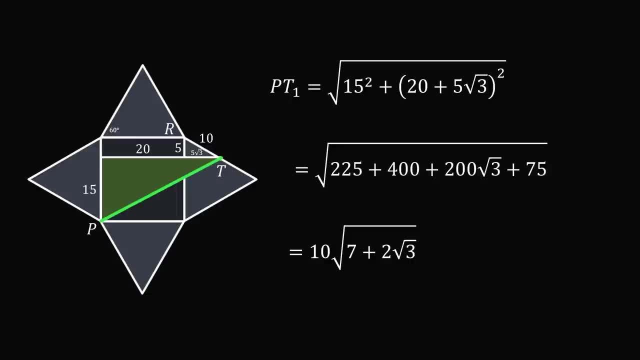 We simplify this to get: pt is equal to 10 times the square root of the quantity 7, plus 2 times the square root of 3, and this is approximately equal to 32.348.. We'll keep this value in mind, and now let's calculate the length of pt in the other case. 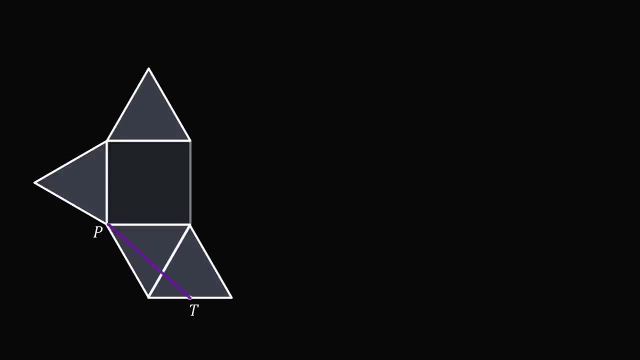 We want to calculate the following length of pt. This is the vertex O. Each edge in this pyramid has a length equal to 20, and then t is along the midpoint, so we know that this length is equal to 10.. Each of the triangular faces is an equilateral triangle, so each of the angles is equal to. 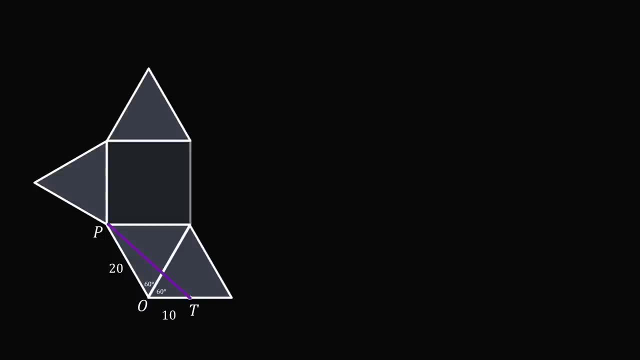 10.. We can now calculate the length of pt using Al-Kashi's Law of Cosines. The length of pt will be equal to the square root of 20 squared plus 10 squared minus 2 times 20 times 10 times the cosine of 120 degrees.